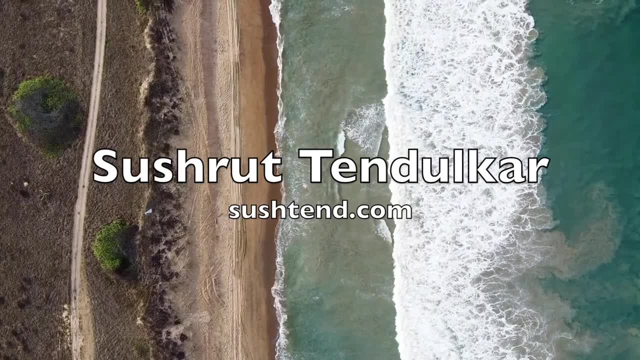 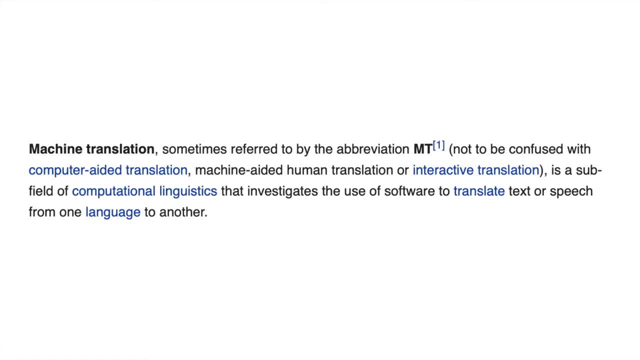 What is machine translation? Well, according to Wikipedia, it's a subfield of computational linguistics that investigates the use of software to translate text or speech from one language to another. When you search in Google about what is machine translation, you'll find that it's. 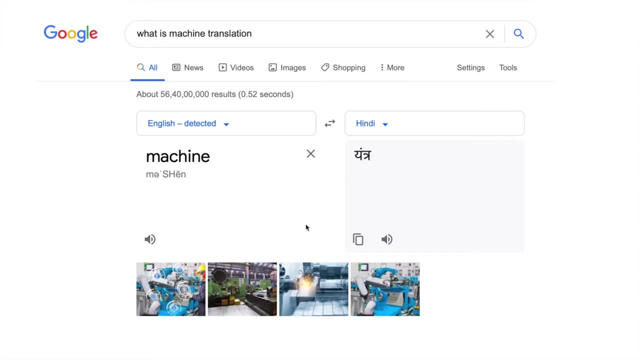 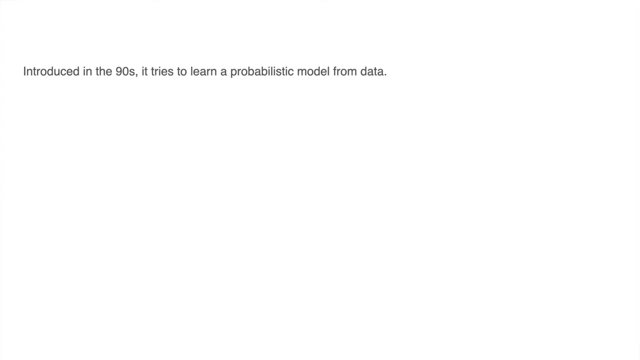 machine translation. This is what you get. Anyways, there are two types of machine translation techniques: statistical machine translation and neural machine translation. Let's see what is statistical machine translation? Introduced in the 1990s, it tries to learn a probabilistic model from the data. Basically, we want to find the best. 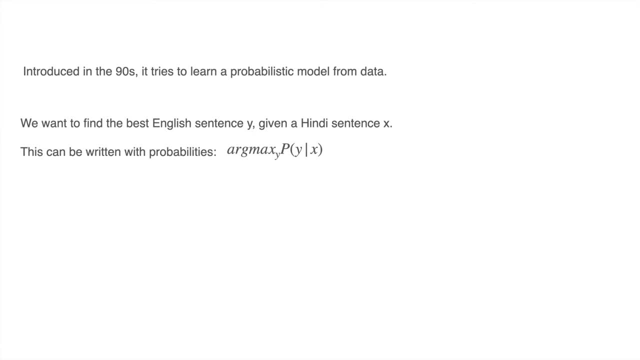 English sentence Y given Hindi as an example sentence X. This can be written with the probabilities as probability of Y given X. So here Y can be any target sentence, X can be any source sentence. Now we can decompose this equation using base rule into probability of Y given X, as: 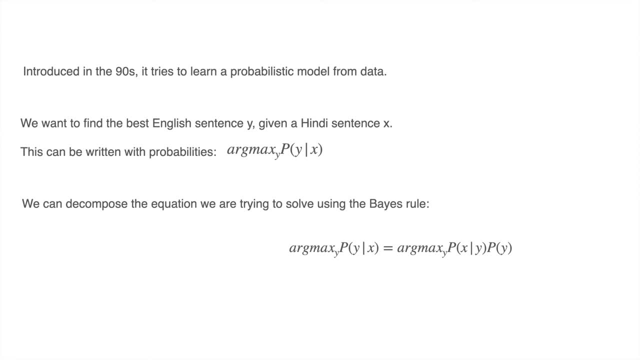 related terms. plus X, What we get is the Similarity Component for Y and Y. The probability of Y is equal to the Translation Model. If we say that X is equal to Y or Y is equal to Y, then probability of Y is the Translation Model, And then we get that Y is equal to Y. So we 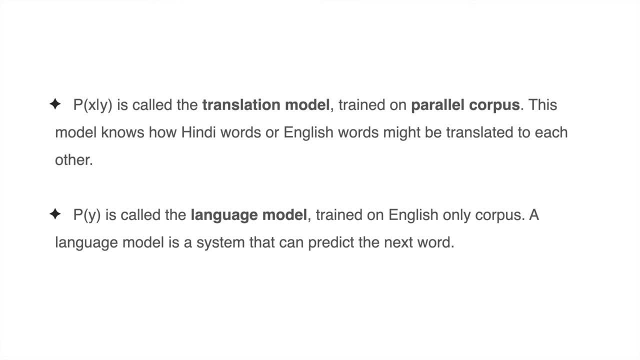 are expected to fill land of text journal as Y. After hamming our declines, we have greater probability of the Y and Y Or playing around. we will get greater probability of Y as equal to Y. We will get greater probability of Y. 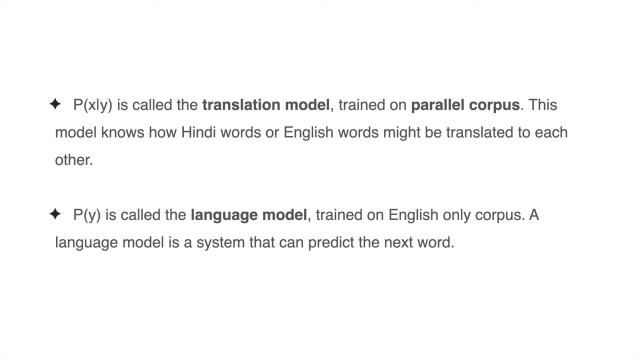 and now I'm going to dólares17203.. Okay, so I just�arlos these. ně 이� KO to each other. and probability of Y is called language model, which is trained on the target sentence. in this case it is English. a language model is a system. 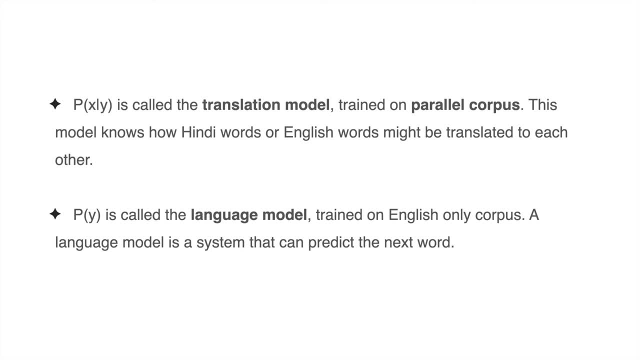 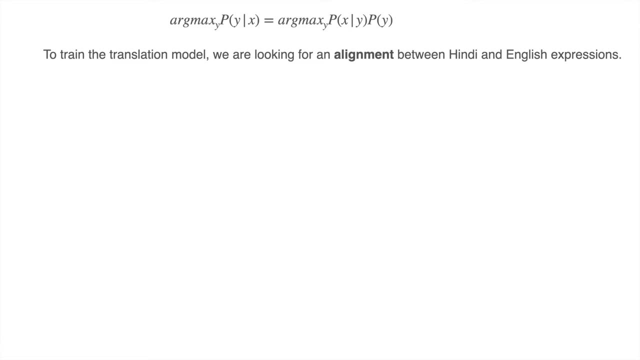 that can predict the next word which we have seen earlier in the series. now to train a translation model, we are looking for some kind of alignment between the Hindi and the English expressions. let's say we have a Hindi sentence- Aap kaise hain- and the English translation, as how are you? now, for each word we have a 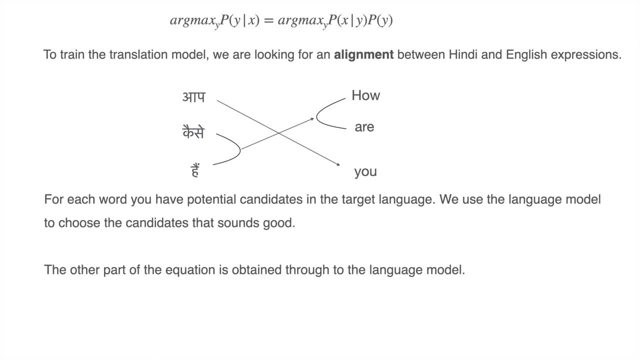 potential candidate in the target language and we use language model to choose the right candidate. the second part of the equation, that is probability of Y, which is a language model that is obtained through training, a language model on the target sentence: here we have Hindi as the source sentence and 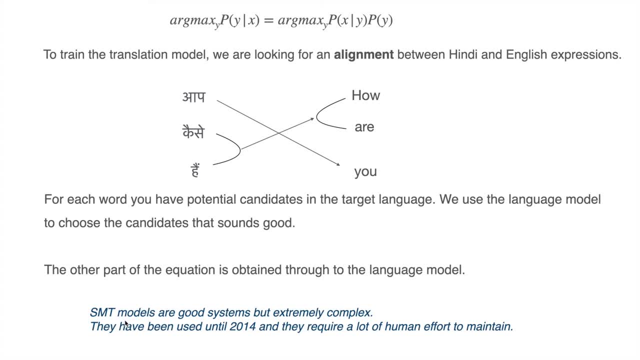 English as the target sentence. statistical machine translation models are good systems but they are extremely complex and they require a lot of human effort to maintain because, as we seen, there is a lot of laborious work of mapping the words from the source sentence to the target sentence and then 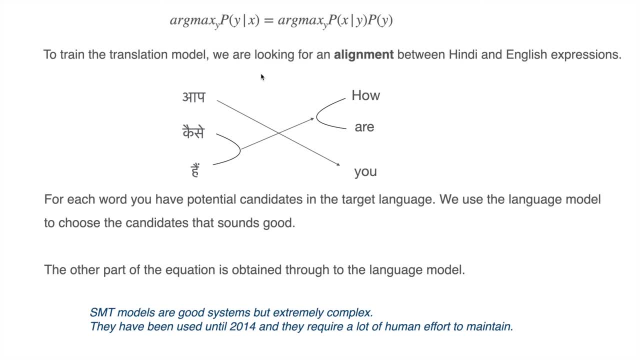 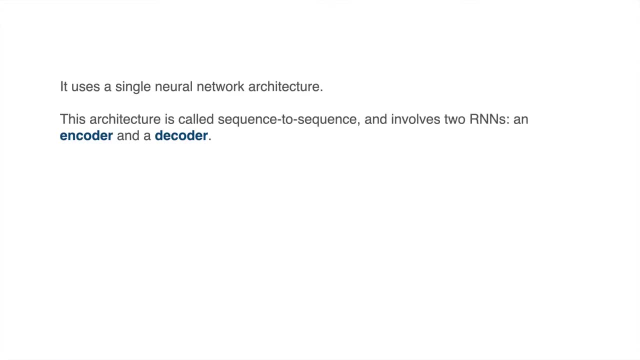 they. they can be used in training this SMT systems- neural machine translation. it uses a single neural network architecture. the architecture is called sequence-to-sequence and it involves two RNN's, or recurrent neural networks. one is called encoder, other one is a decoder. the encoder will produce the encoding of 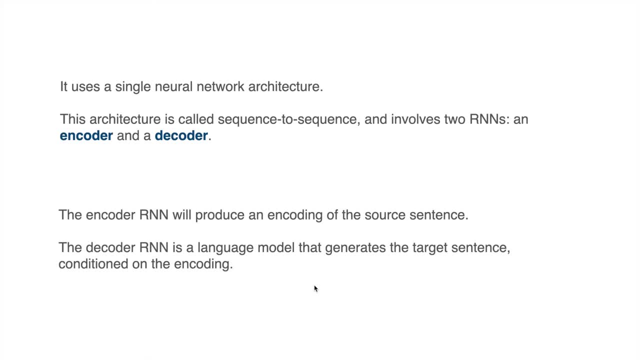 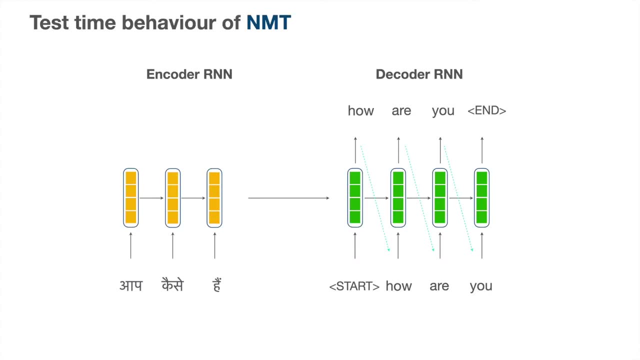 the source sentence and the decoder will produce the target sentence based on the conditions of the encoding. let's see an example. imagine we have already trained an empty systems and this is how it would behave in the test time. At different time steps we provide the words from the source sentence and the last hidden. 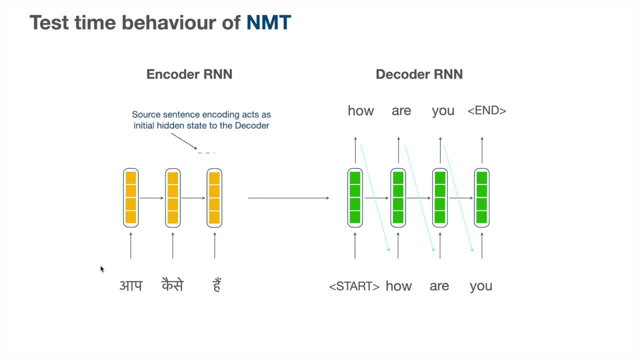 state will have the encoding of this entire sentence And this encoding acts as the initial hidden state to the decoder here And this will produce output. the first output, how, and that will be directly fed into the next hidden state. that will produce the next word, are, and that is again fed into the next. 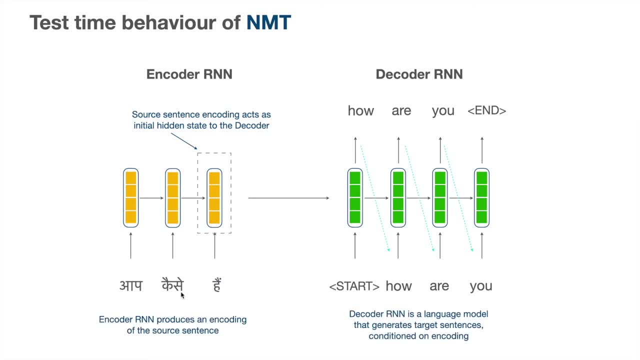 hidden state and it continues. As you have already seen, the encoder RNN produces the encoding of the source sentence which is available at the last hidden state, and the decoder RNN is a language model that generates the target sentence conditioned on the encoding. This is a simple example of the encoding of the source sentence. 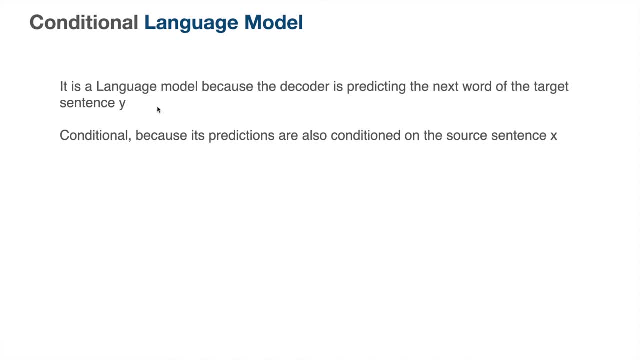 It is a conditional language model. because it is a language model because the decoder is predicting the next word of the target sentence, y. It is conditional because its predictions are also conditioned on the source sentence, that is, x. Unlike statistical machine translation, NMT directly calculates probability of y given. 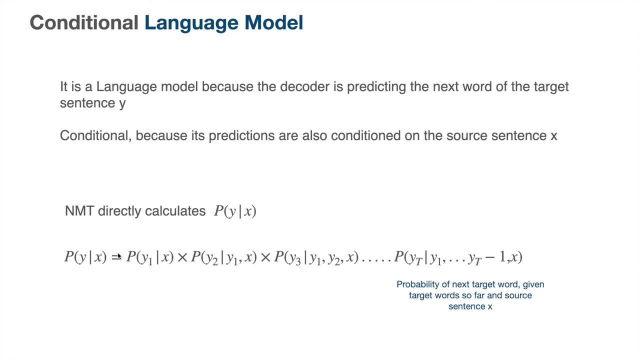 x, that is, probability of y1 given x times probability of y2 given x. So here y1 is the first predicted word. this is the second predicted word, given the first predicted word and the source sentence. Here the probability of the third word, third predicted word, given the already predicted 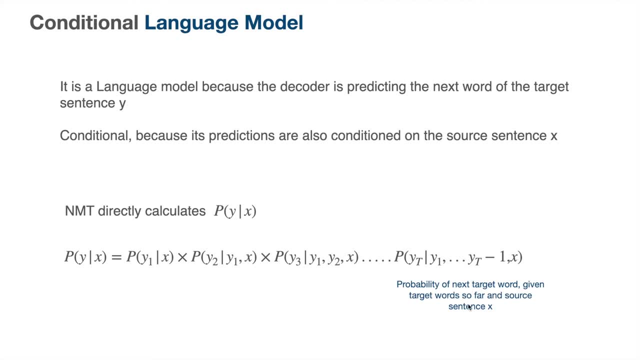 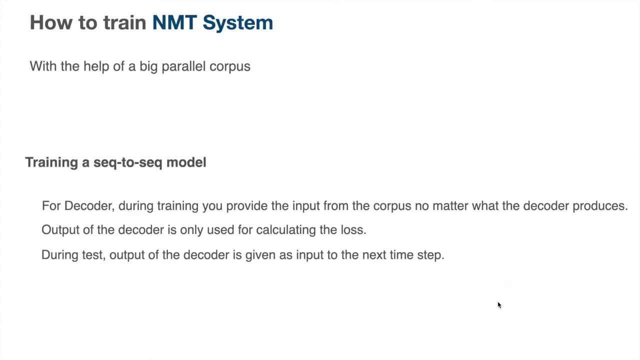 first and second word and the source sentence and it continues. So basically it is probability of the next target word, given the target word so far and the source sentence x Now how to train an NMT system. We need to have a big parallel corpus. 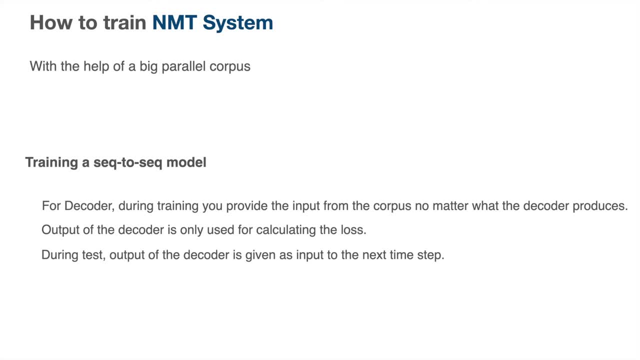 What is a parallel corpus? Its collection of parallel sentences from both source as well as the target language. Now how do you train a sequence to sequence model? What we have just seen is the test time performance of an NMT system. Now, to train a sequence to sequence model, we need to provide the input from the corpus. 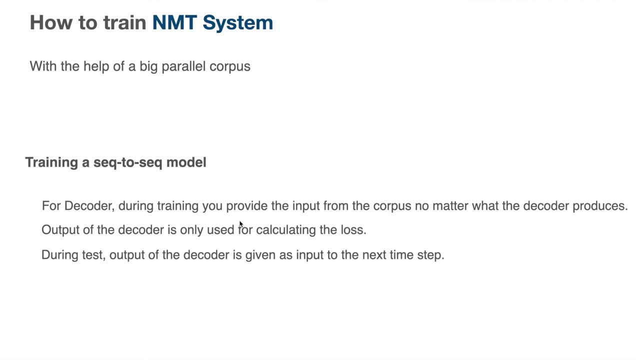 no matter what the decoder produces. So during training We use The output of the decoder for calculating the loss and we are not going to feed that into the next hidden state. we are going to use the output of the decoder to calculate the loss and update the weights. 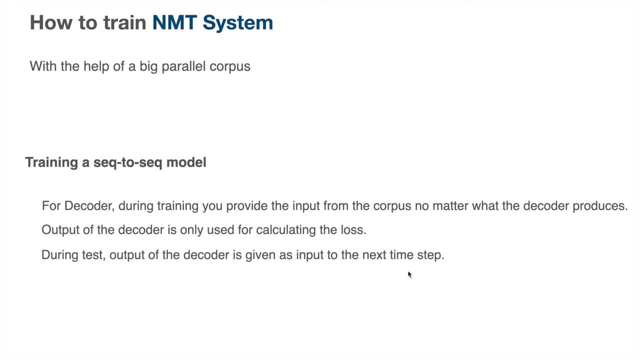 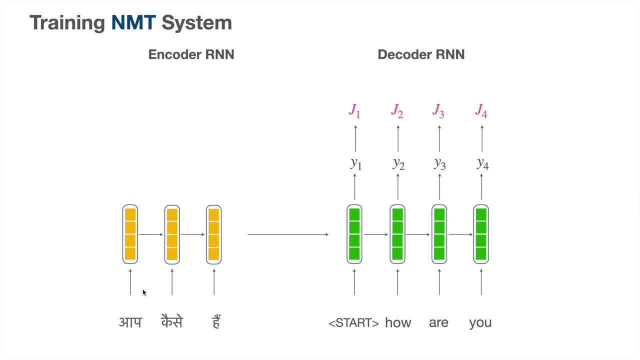 But during the test time the output of the decoder is directly given as input to the next time step. Let's look into the training process of the NMT system. We feed the source sentence at different time steps and that is encoded at this last hidden. 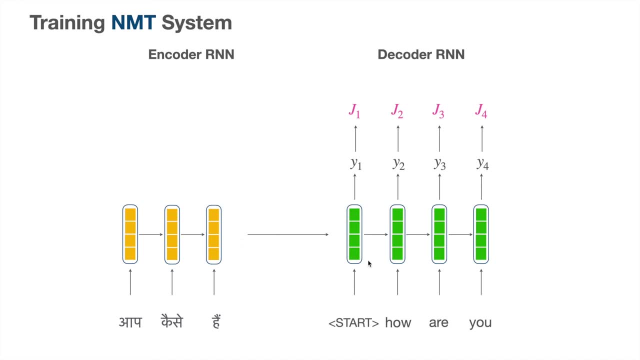 state And that acts as an input for the decoder, which will produce the first word, Y1. And we calculate the error here, which is J1.. So J1 is nothing but the negative log probability And we have also seen the error function, the calculation of the error function and